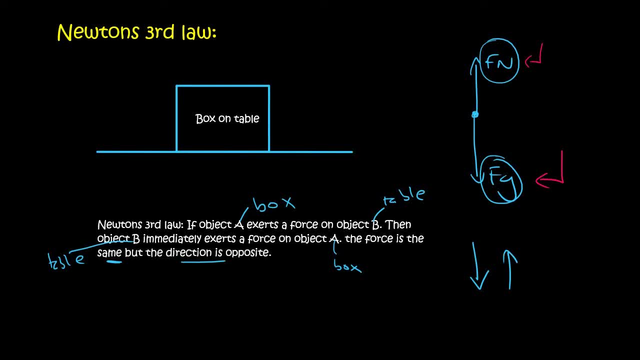 a force on the table and the table is exerting a force on the box. If you had to look at the force, they would be the same. It would be five newtons, for example, and five newtons So Newton's. 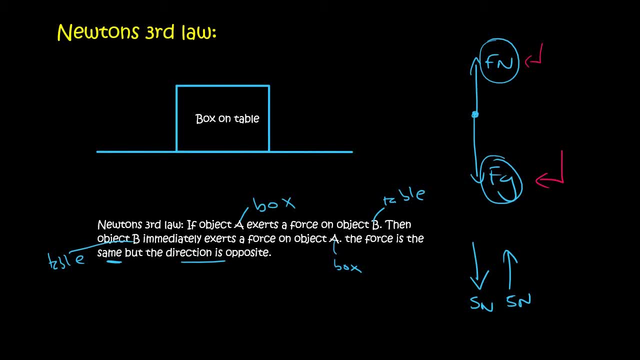 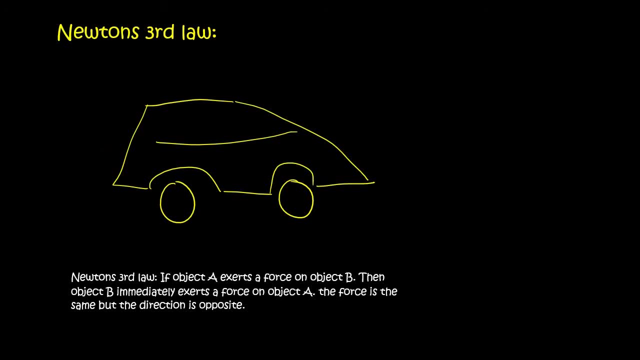 third law is about objects that are acting on each other. The force is the same, but the direction is opposite. So let's say we have a car that is busy driving and it collides with a little fly. Okay, so let's say there's a fly and that fly collides with the windshield of the car. 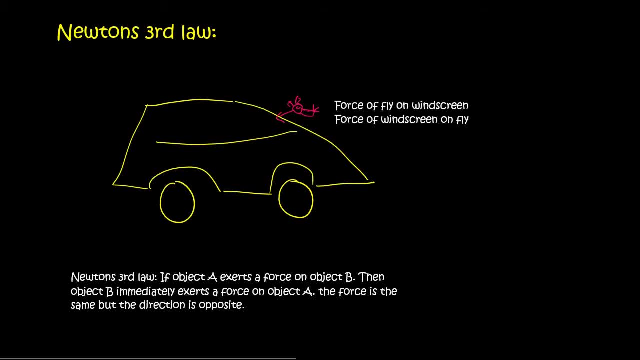 Then we have two forces present. You would have a force of the fly on the windscreen. So if I had to draw the windscreen, that windscreen is going to feel a force from the fly, But then if you have to draw the fly, then it will feel a force due to the windscreen. Now can the words be switched? 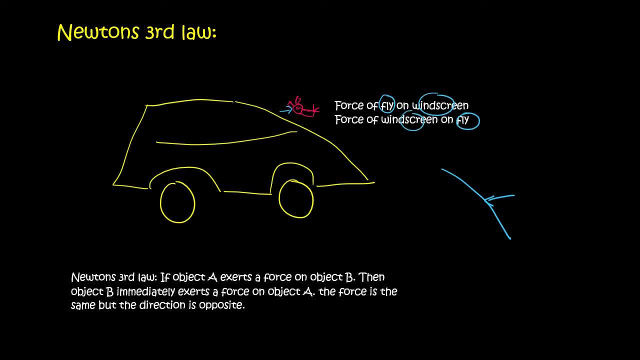 Well, here we've got fly and windscreen, and here we've got windscreen and fly. And so, yes, this is a Newton's third law pair. So it tells us that the force is the same on both objects, but the direction is opposite. Okay, but then, Kevin, why does the fly get? 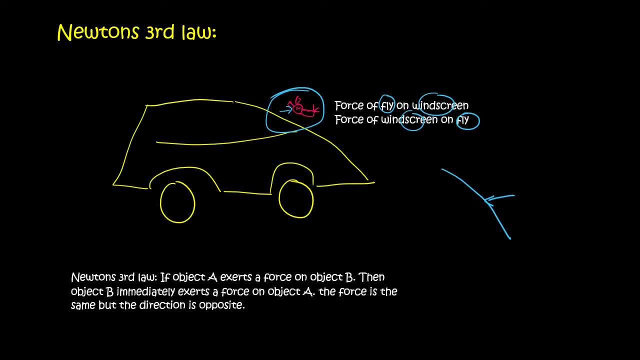 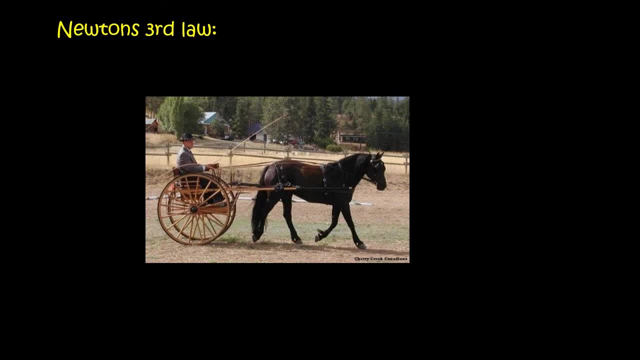 completely destroyed and the car barely feels a thing. It's due to the mass. The mass of the car is a lot larger and the fly is obviously a lot lighter, And so the fly will undergo a much larger acceleration, and that's what causes the damage. So if we had to look at this system over here, 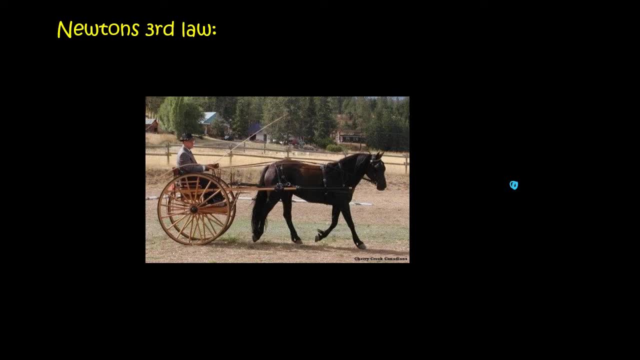 let's draw a free body diagram on the horse. So obviously the horse has its own applied force. There's a normal force which is keeping the horse up, Then there's the force of gravity acting on the horse, Then there's a backwards force. Let's say there's no friction. 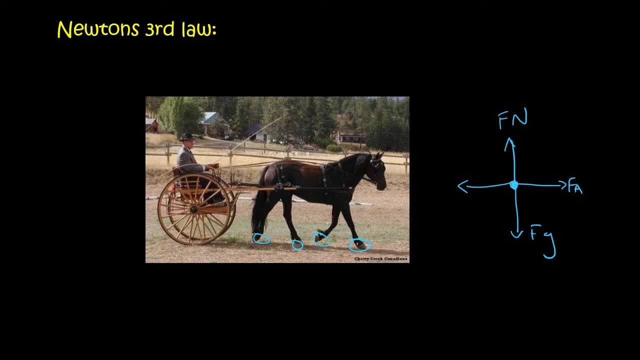 by the hooves. But let's say there's a tension force, or let's say there's the- I'm going to call it FC- for the cart, Then I'm going to do a free body diagram on the cart, And so that's going to have gravity, That's also going to have some friction at the wheels. 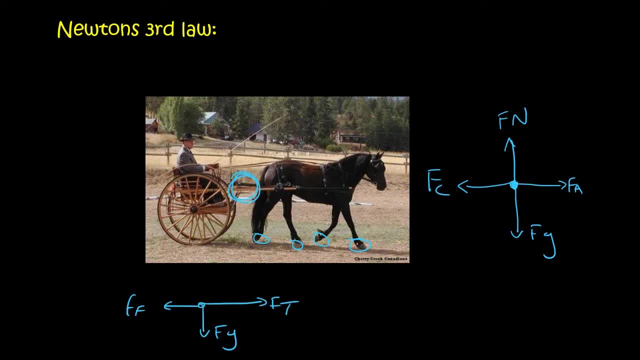 Then there's going to be a tension force, which is due to the horse over there, And then there's a normal force that is keeping the horse, that is keeping the cart upwards, And let's just assume that this person doesn't exist. Okay, so you get out of here. Now we need to try identify a Newton. 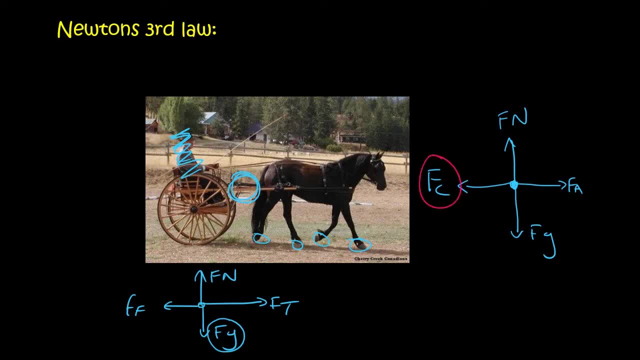 third law pair. Now, what many people say is they'll say: okay, well, these two are a third law pair. Well, let's look at that carefully. This is the applied force of the horse And this one is the force of the cart on the horse. So, guys, those are not. 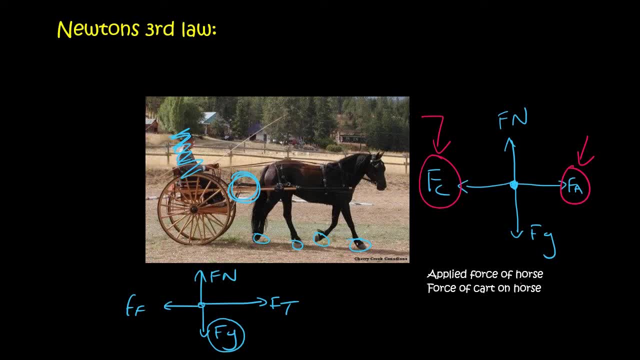 a Newton third law pair. Look at this. This is the force applied force of horse And this is force of cart on horse. There's no similarities there at all. The next one people say is the normal force and the force of gravity. Well, the normal force is the following: Normal force is: 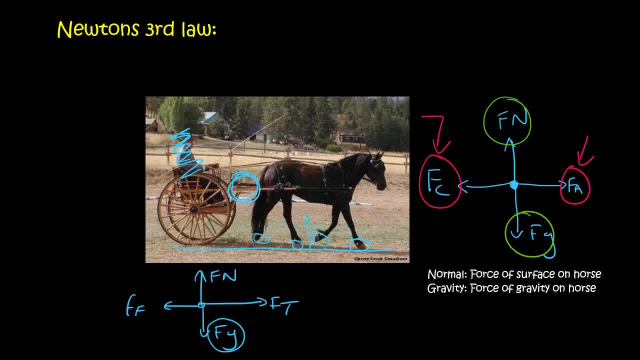 the force of the surface, So it's the ground that is exerted on the horse. Gravity is force of gravity on the horse, So both of those are acting on the horse. With a Newton third law pair, it has to be two different objects exerting forces on each other. 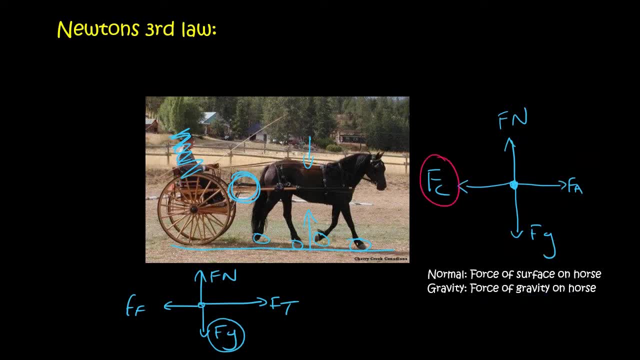 Now I'll show you what I mean by that. now, If we look at the cart, then that- or in fact it would be better to call it FT, Because it's the force of tension in this pulling piece on the horse- 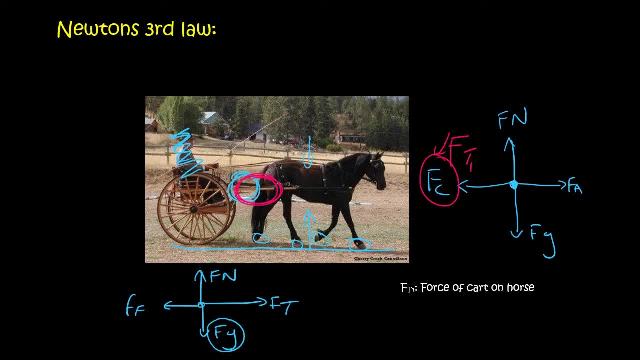 And I called it FT1.. Let's call it FT1.. And then this one is FT2.. Now let's look at what FT2 is. That is the force of the horse on the cart. Now we have Newton's third law Cart on horse and horse. 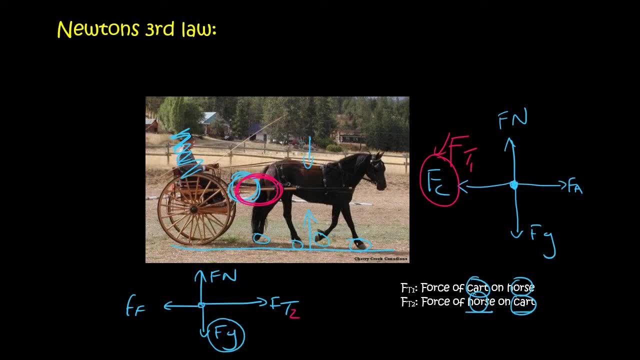 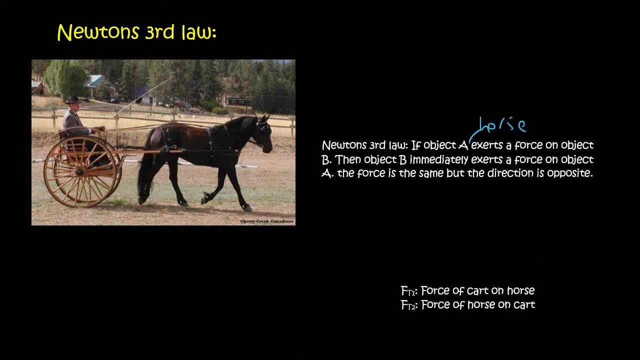 on cart. If you can switch them like that, then it's a Newton's third law. And remember what Newton's third law says: If an object A, such as a horse- let's say that's the horse- exerts a force on, 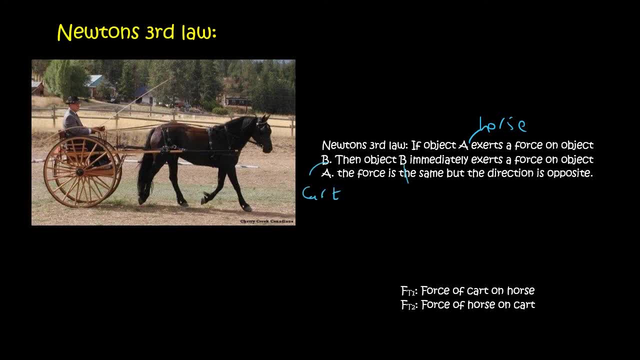 object B, which is the cart, then object B, which is the cart, immediately exerts a force on object A, which is the horse. The force is the same, but the direction is opposite. So if the horse is exerting 10 Newtons on the cart, then the cart is exerting 10 Newtons on the horse. So what that? 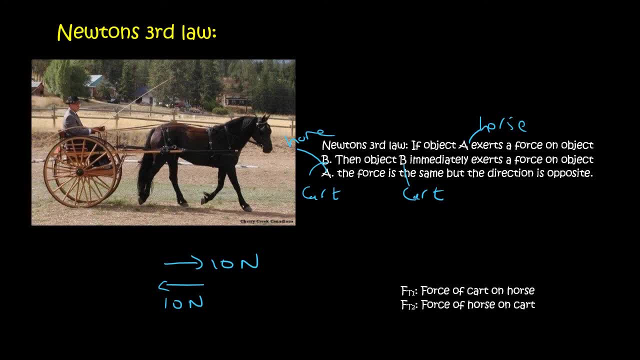 means is that if this horse decides that it really wants to start speeding up, then it's going to increase the force that it exerts on the cart, But then at the same time the cart's force is going to become larger as well. So it's almost like: imagine you've got. 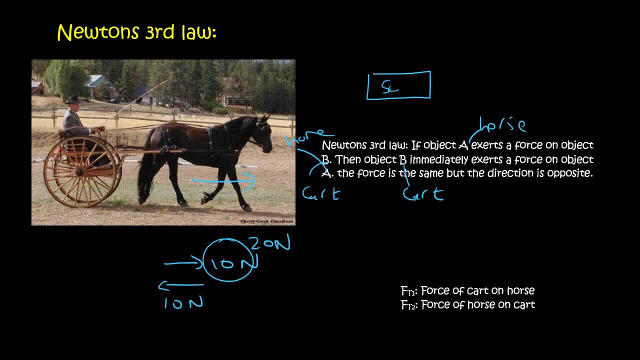 a bag, a heavy, heavy bag, like a 50 kg cement bag. If you are pulling that along the floor, if you pull it very slowly, then that means that your force applied is relatively low. If you decide that you want to get the job done faster, then you start.